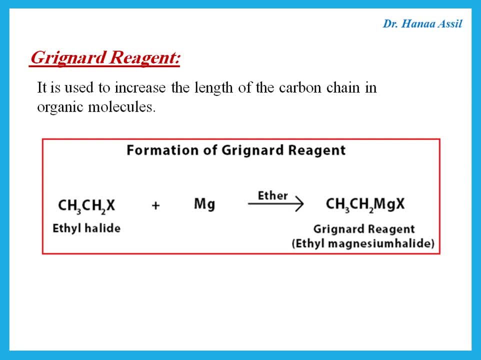 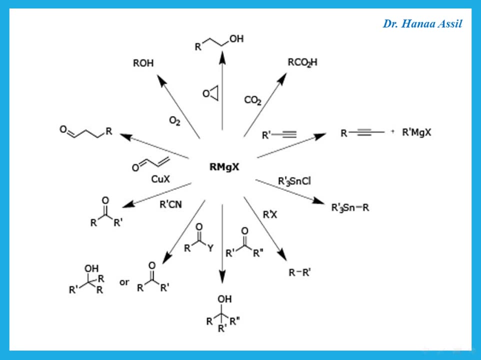 halide to form what we call a grignard reagent. So in this case it's called, for example, ethyl magnesium halide. Okay, and then we use this grignard reagent to react it with a wide range of compounds in order to prepare many different types of organic compounds. So let us take a look. 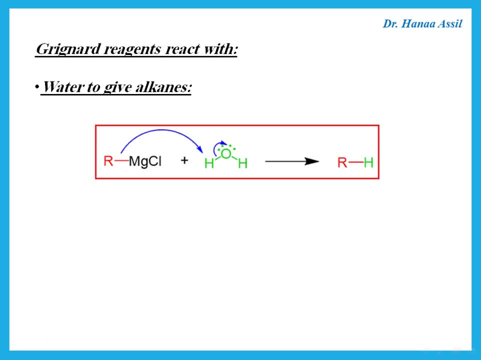 at this one by one. How do I use grignard reagent? The grignard reagent: if I want to prepare an alkane, I react it with an alkyl halide. So I take a look at this one by one. 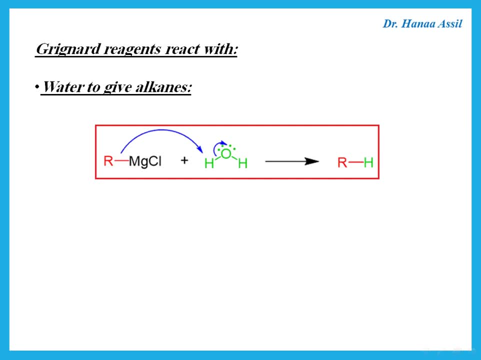 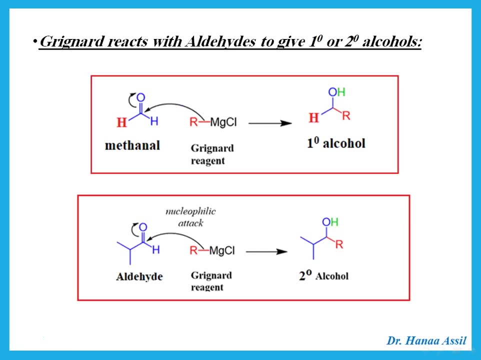 So to prepare an alkane. the grignard reagent reacts with water. When we react it with aldehyde it will give either the primary or the secondary alcohol. So if I react it with methanol it gives the primary alcohol. If I react it with any other aldehyde, then it will give a secondary. 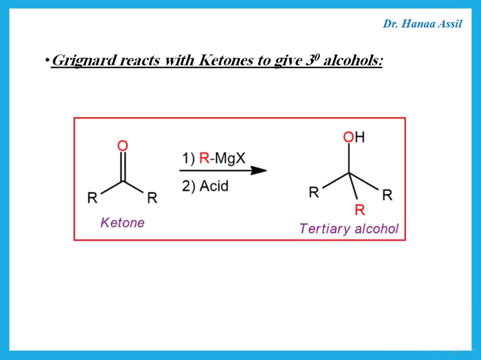 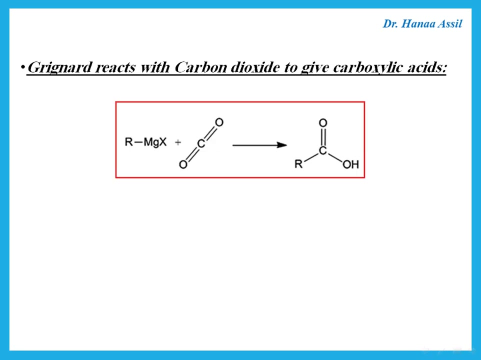 alcohol. Now, when we react it with ketones, then it gives a tertiary alcohol. So grignard reagent with a ketone will give a tertiary alcohol. Are we following? Okay, what if I react it with something like carbon dioxide? Now if I react grignard reagent with carbon dioxide, what we get is: 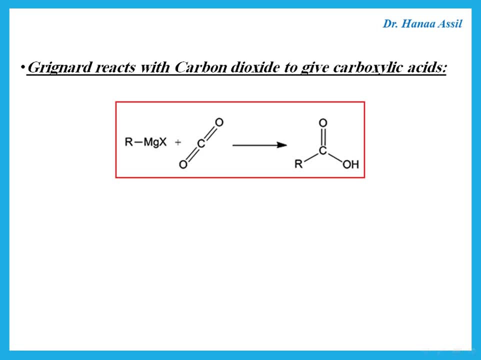 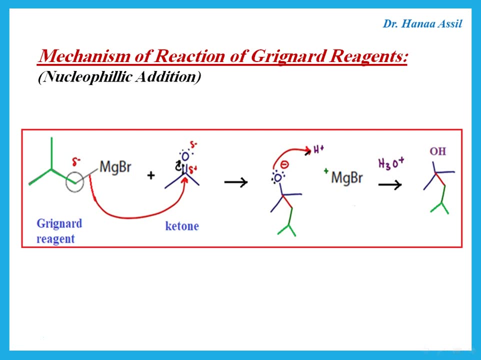 an acid. So in order to prepare a carboxylic acid, I need to react the grignard reagent with carbon dioxide. How does the grignard reagent work? It works with nucleophilic addition. So the grignard reagent, the carbon that is attached to the magnesium bromide, or magnesium. 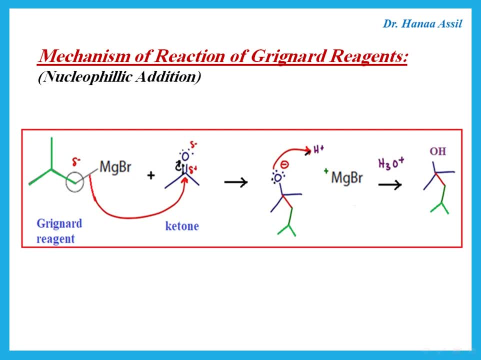 chloride. this carbon is a slightly negative carbon So it acts as a nucleophile that attacks a carbonyl carbon. If it is reacting a ketone, we said it gives a tertiary alcohol. So the grignard reagent reacts with nucleophilic. 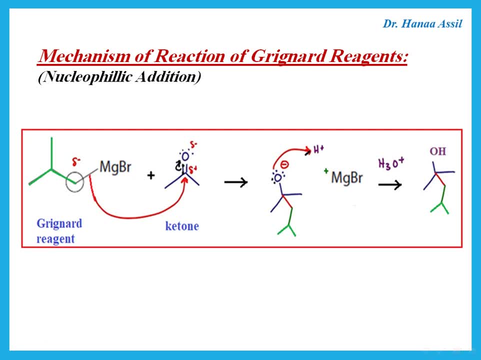 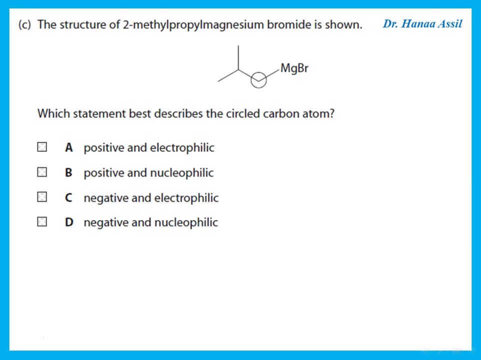 addition, The carbon- slightly negative carbon- acts as a nucleophile that attacks the slightly positive carbonyl. In the end, in this case it gives a tertiary alcohol. So let's take a look at this question. The question says the structure of 2-methyl propyl. 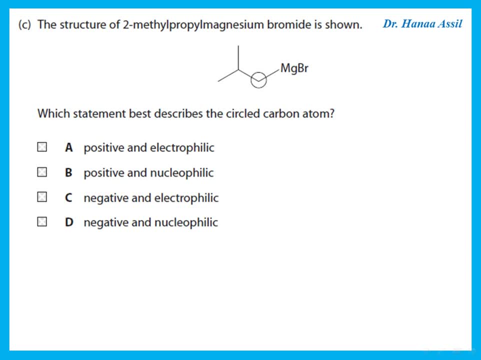 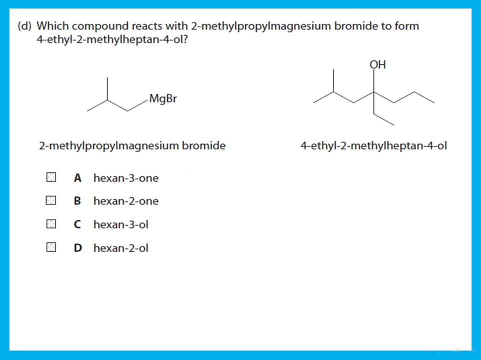 magnesium bromide is shown. Which statement best describes the circled carbon atom. We said this carbon atom that is attached to the magnesium bromide. it acts as a nucleophile- negative, slightly negative carbon and the reaction is nucleophil. which compound reacts with two methyl propyl magnesium bromide to form four ethyl 2-methyl? 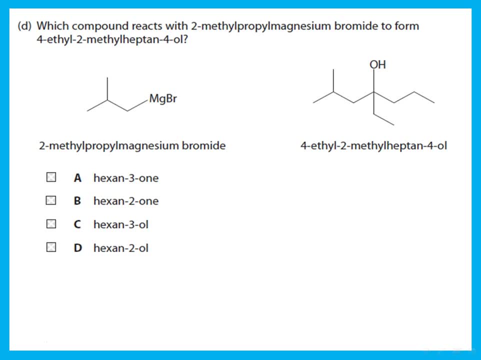 heptane for all. so he gives me the compound i'm trying to prepare using this greenery agent. so, looking at it, you should realize that this is the new part that i am adding to the greenery agent. so it's as if i am removing the magnesium bromide and putting that chain instead of it. so what? how? 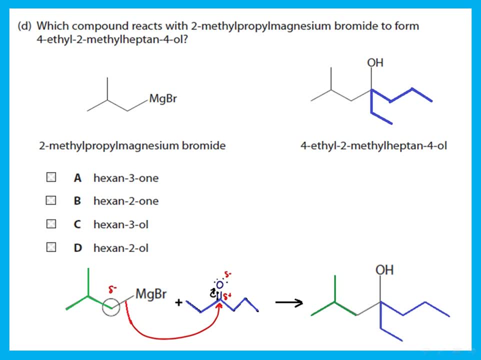 do i react it or what do i react it with? i have to react it with this ketone in order to get that part added, so that ketone is hexane three ohm. can you see how we think about it? let's see the part we're adding. 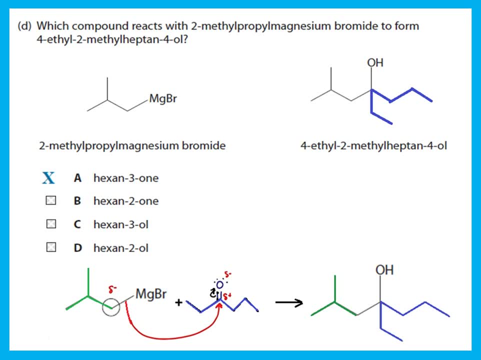 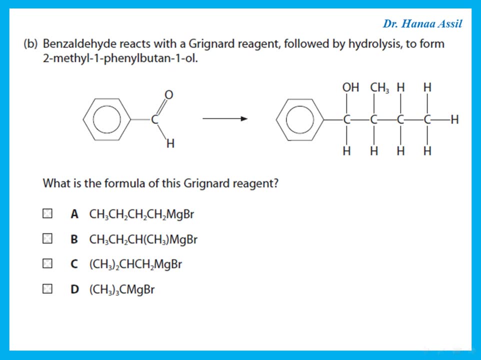 and then we put it as a ketone or an aldehyde, if that's what it was. benzaldehyde reacts with a greenery agent, followed by hydrolysis, to form this compound which we call two methyl, one phenyl butane one all. what is the formula of this greenery agent? now, he's. 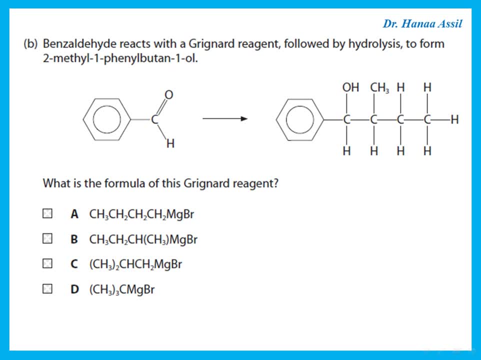 going to look at it and he wants to know which one is the greenery agent. so if we look at it, this is the part that we have from the benzaldehyde, so the rest of it is the part that we get from the green yard, so the rest of it with a magnesium bromide, that is my greenery agent. so which one is? 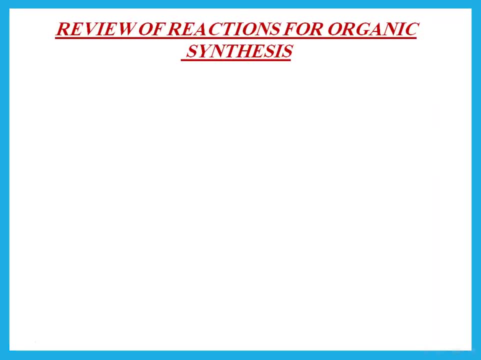 the correct answer. you can see that is the correct answer. and then we go through a very quick review of the chemical reactions, that many of the chemical reactions that we will need in order to repair organic compounds in this syllabus. so let's take a look, for example, if i have a benzene ring, we talked about benzene ring and we said, if i want, 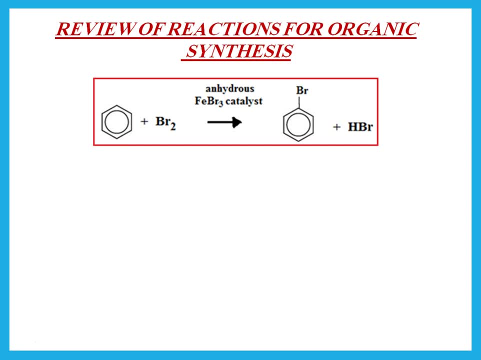 to add a halogen to the benzene ring. i react it with uh, the halogen in presence of anhydride rose febr3, or it could be chlorine in anhydrose, fecl3 as a catalyst. so that's one useful reaction we're going to use. another reaction is if i want to put a methyl group on the benzene ring. 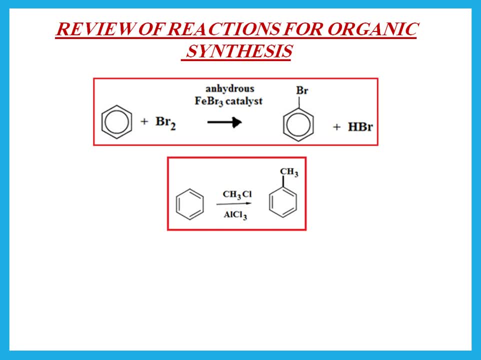 how do i react? it remember that to add a methyl group. this was what we call friedel kraft's alkylation. so we reacted with methyl chloride in presence of aluminum chloride. what if we have the methyl benzene and i want to add a chlorine on the benzene ring? 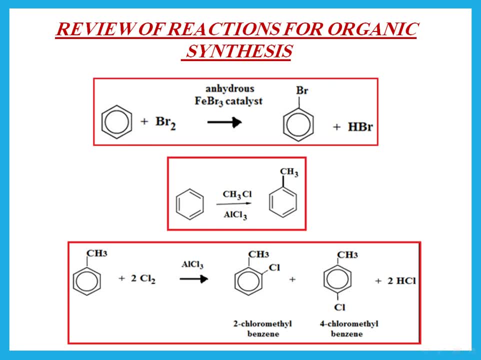 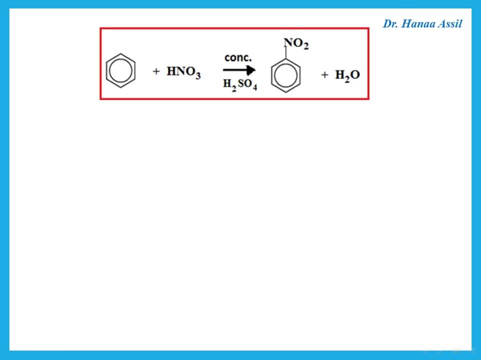 in that case we react it again with chlorine in presence of aluminum chloride, like that first reaction, and remember that if i have a methyl group then i put the incoming chlorine either on carbon number two or on carbon number four. this is another useful reaction that we talked about and we will need it to prepare organic 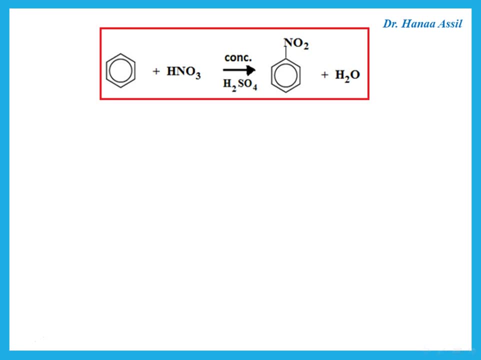 compounds. how do i put a nitro group on the benzene ring? if i have a benzene ring, i need to react it with what? concentrated nitric acid, concentrated sulfuric acid? then it puts an no2 group on the benzene ring. so this is how we make nitro benzene. 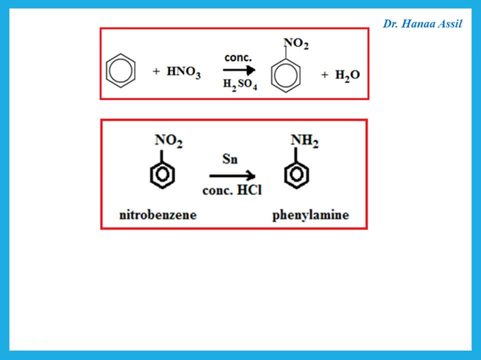 then if i want to change the nitro benzene to an amine- phenol amine- i need to change the no2 on the benzene ring. i need to make an amine. then i react it with 10 in presence of concentrated hcl. 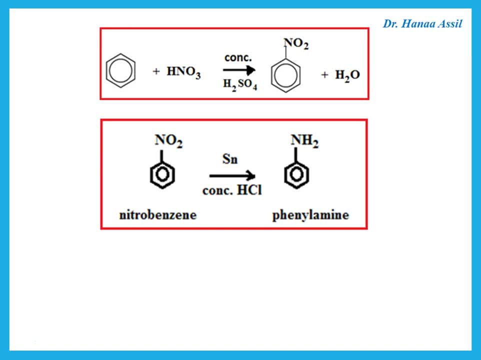 do you remember all of these reactions? so please, uh, remind yourselves of all these reactions. we're going to need it for the organic synthesis schemes. so if i have a nitro benzene and a phenol amine with have a methyl benzene and I want to oxidize the methyl group so that I get, 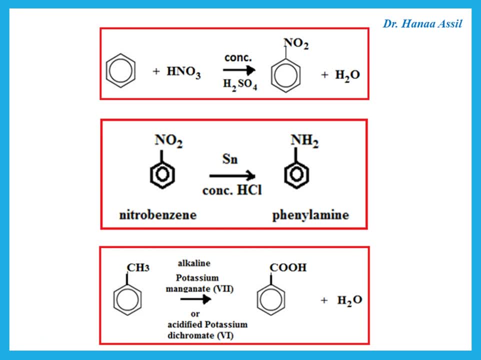 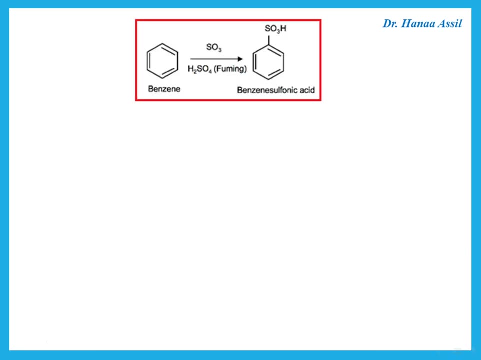 the acid. so to make benzoic acid, for example, I need to react the methyl benzene with alkaline, potassium, manganese or acidified potassium dichromate. what if I want to put a sulfonic group on the benzene ring? in that case I react the benzene with what we called fuming sulfuric acid. 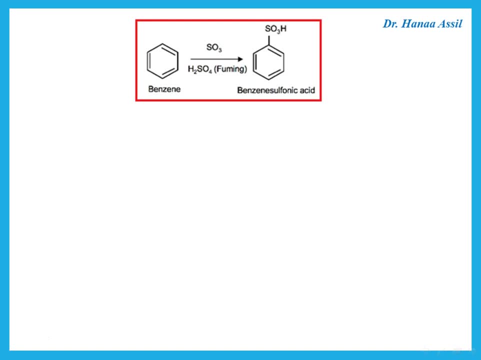 which is sulfuric acid, with sulfur trioxide. this will put the SO3H group on the benzene ring. what if I want to prepare a nitrile? remember we said we need what we may need- a nitrile in order to add a new. 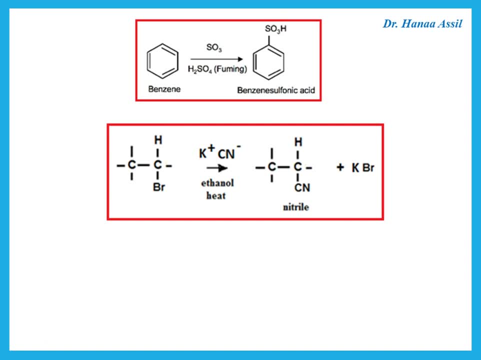 carbon to the chain. so from the halogen alkene I can react it with potassium cyanide in ethanol. this puts a nitrile group, a cn group, on the benzene ring. so i'm adding an extra carbon. what if i want to prepare an amine? we said: how do we? 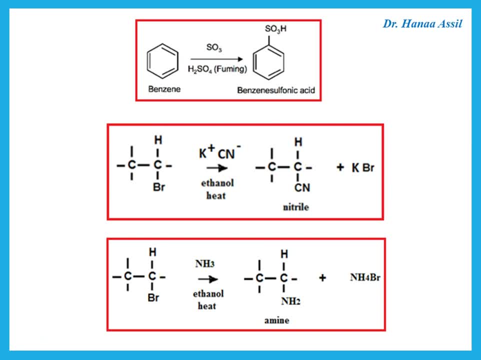 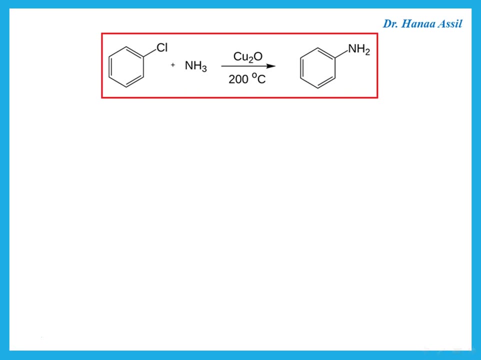 prepare amines, we react the amine with a halogen alkane. so a halogen alkane in presence of ammonia in ethanol. this will replace the halogen with an amine group. okay, what if we're trying to make phenol amine from chlorobenzene? so i have a chlorine on a benzene ring and i want to replace. 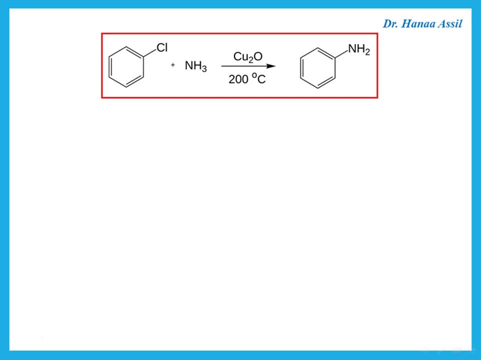 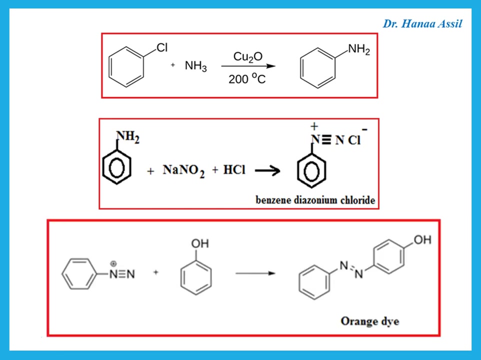 it with the amine group. we said we can react it with ammonia, this phenol amine. we can use it to make benzene diazonium chloride. and we said, to change the nh2 to a diazonium chloride, we react it with sodium nitrite in hcl. and then this benzene diazonium chloride i can react it with. 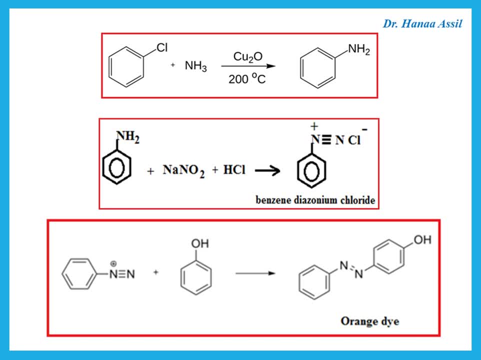 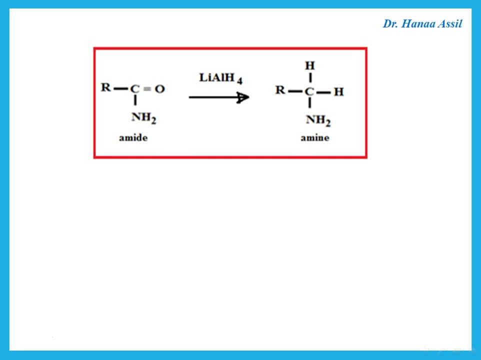 something like phenol in order to make an azo dye, which we said is a colored dye, orange or yellow- reaction of amide. remember, we did amides and we said: okay, if i want the amide to become an amine, i can react it with lithium, aluminium hydride and this gives me the corresponding amine. 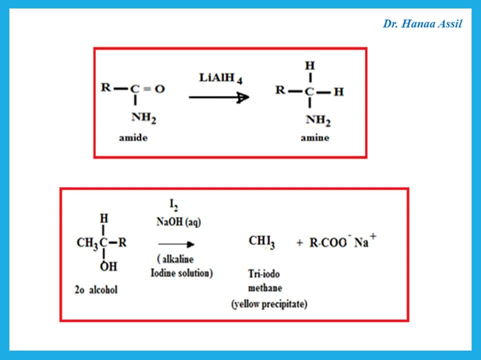 if i react a secondary alcohol and i want to remove one of the carbons, this is how we remove a carbon from a chain. so if i'm starting with two carbons and our or certain number of carbons and i want to remove a carbon, then i can react it with iodine in sodium hydroxide. so this is alkaline iodine solution. 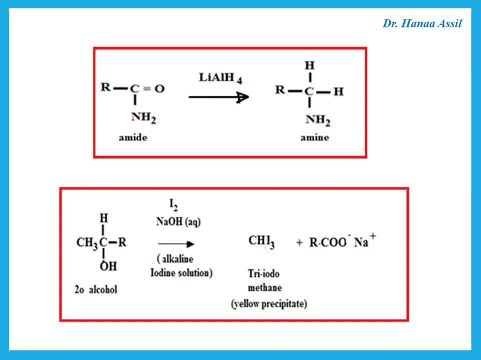 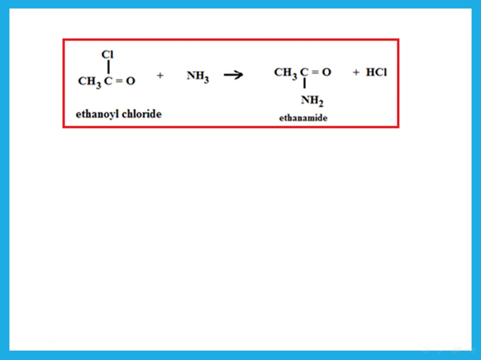 this reacts if we have a secondary alcohol so that we have the group ch3, coh, then the ch3 is removed and i end up with the sodium salt of the rest of the chain, ethanoil chloride. we said ethanol chloride is very useful. i can react it with ammonia if i want to. 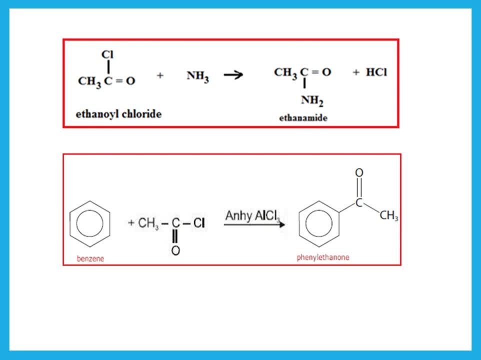 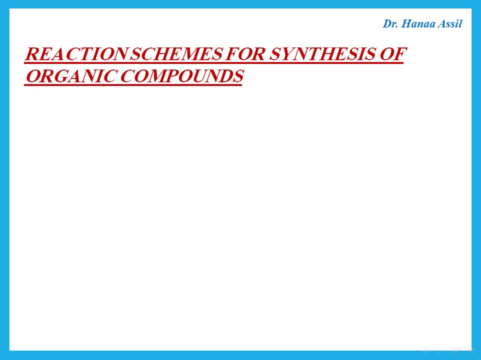 make a thanamide, or i can react it with benzene if i want to add this group to the benzene ring. so this is phenol ethanol, and we can use all of these reactions, and there are other reactions, actually, that we may be talking about. 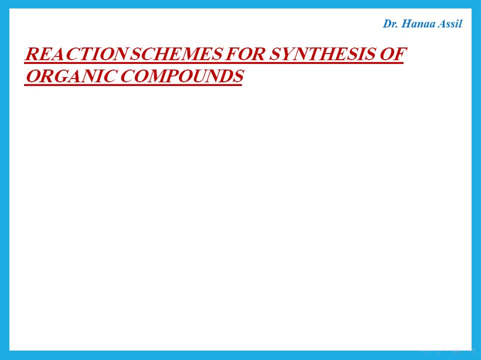 in order to devise reaction schemes for synthesis of organic compounds. So let's take examples of this, And in this syllabus we need only up to four steps in order to prepare organic compounds, so we don't have very long reaction schemes. But let's take a look at shorter reaction schemes. 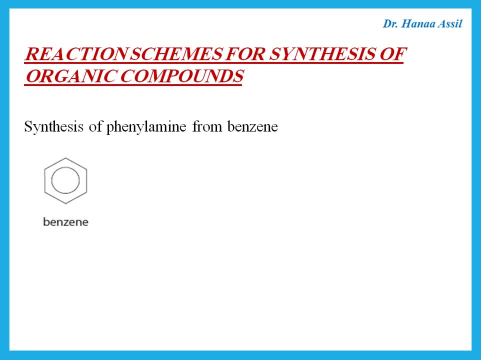 First. for example, if he says: I am trying to prepare from benzene, I want to make phenyl amine, Can you see how we think about it? He's saying: I want to make phenyl amine from benzene. 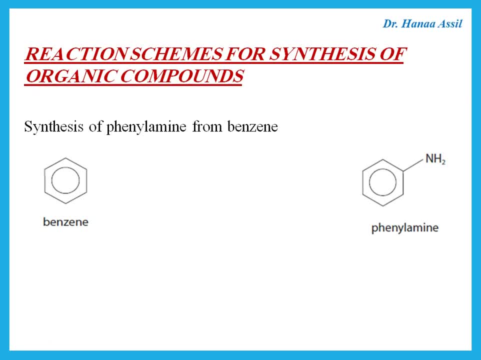 How do we change benzene to phenyl amine? We said actually we can do that directly or we can change it. We can change it into a nitro group first and then change it to an amine. What do we do to the benzene to put a nitro group on it? 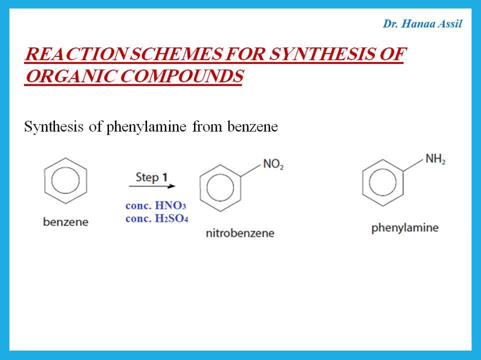 Concentrated nitric acid in presence of concentrated sulfuric acid. This will put a nitro group on the benzene And then I can reduce this nitro group to form an amine. What do we do? Tin in presence of HCl? 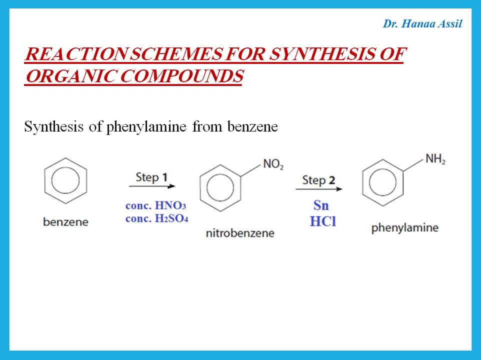 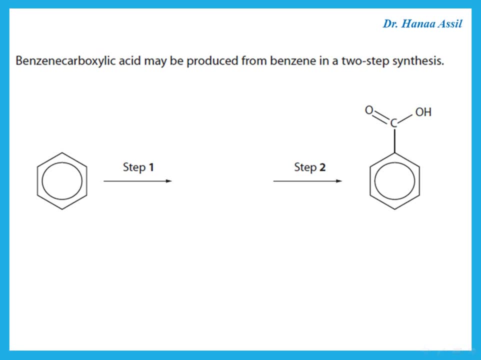 We'll change the nitro benzene into phenyl amine. Let's try another one. In this case, we're trying to make benzene carboxylic acid from benzene carboxylic acid. This is actually benzoic acid. 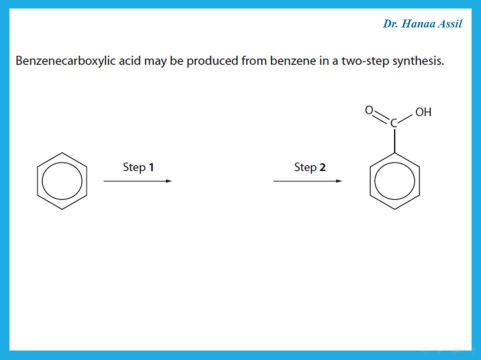 Maybe produced from benzene in a two-step synthesis. So what should we do to change the benzene to benzoic acid or benzene carboxylic, Benzene carboxylic acid? Okay, let's try this First. if I add methyl chloride in presence of aluminum chloride, 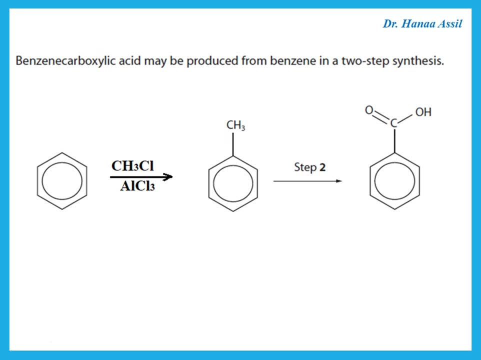 what does that do? It adds a methyl group on the benzene ring. And then we said: what do we do to oxidize the methyl group on the benzene ring to acid? Well, this is alkaline. potassium manganate will change the. 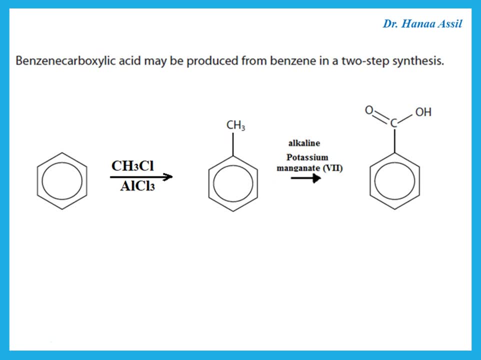 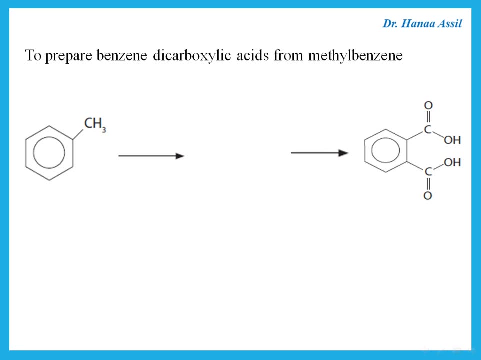 Methyl group to the carboxylic acid group. on the benzene ring Again, if he says: I want to prepare this dicarboxylic acid from methyl benzene, So we're starting with methyl benzene and I want two carboxylic acids. 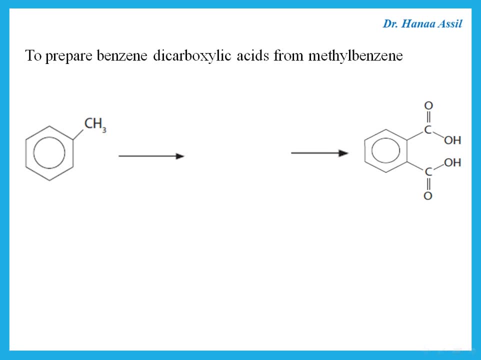 So what can we do? We can first add another methyl on the benzene ring, So react it with methyl chloride In presence of aluminum chloride. this puts another methyl group on the benzene ring, And then we can oxidize this using alkaline potassium manganate. 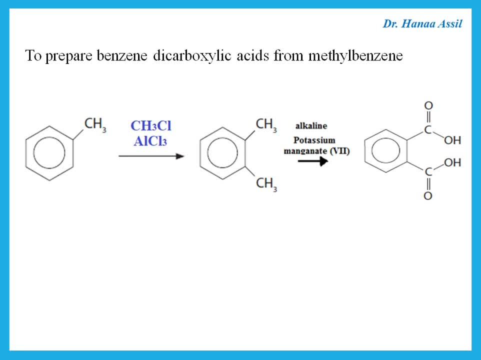 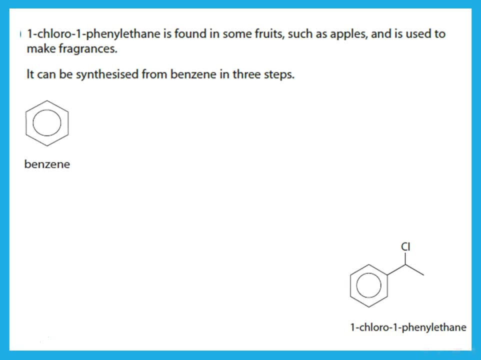 This will put two carboxylic groups on the benzene ring. I want you to know that for all of these schemes, or for most of these schemes, we can have more than one answer to the synthesis. We can synthesize these things in more than one. 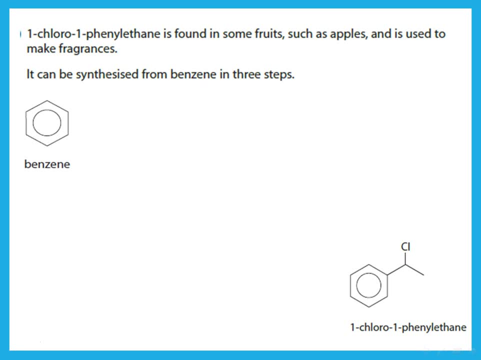 So let's take a look at this example. This is trying to prepare one chloro, one phenyl ethane, from benzene. So he's saying one chloro, one phenyl ethane is found in some fruits such as apples, and is used to make fragrances. 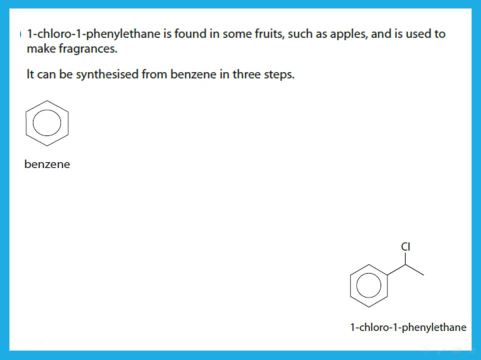 It can be synthesized from benzene in three steps. So what can we do? I want to put this side group on the benzene ring. So what? What do I start with? I can start with ethanol chloride in presence of anhydrous aluminum chloride. 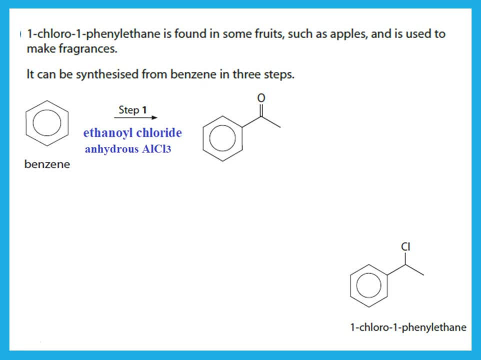 This will put this group on the benzene ring. Remember, Reaction of benzene with ethanol chloride will add this group to the benzene ring. I want to change that to the chloro form. So what can I do? I can reduce the keto to an alcohol. 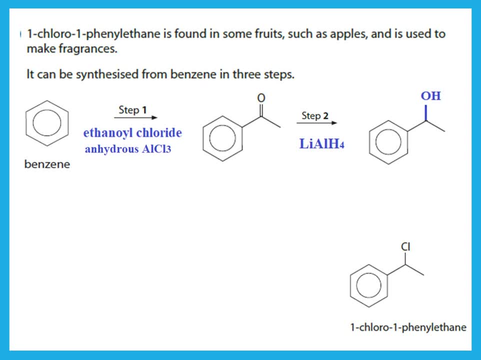 So I put lithium aluminum hydroxide In presence of ether And then we put change the OH to a chlorine. So this is reaction with phosphorous pentachloride, PCL5.. This will exchange the OH with a Cl. 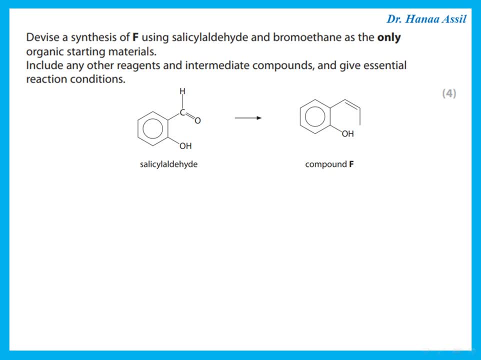 Again. let's try this. He's saying: devise a synthesis of compound F using salicyldehyde- which he already gives me, And bromoethane as the only organic starting material. So he wants you to use this and bromoethane in order to get compound F. 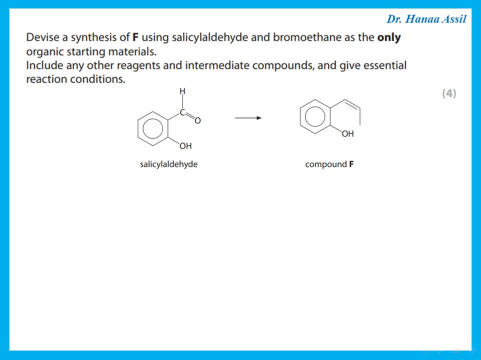 Include any other reagents, intermediate compounds and essential reaction conditions. So what can we do? We have this starting compound and I want to add this group to it. Can you see how we think about it? What are we trying to add? 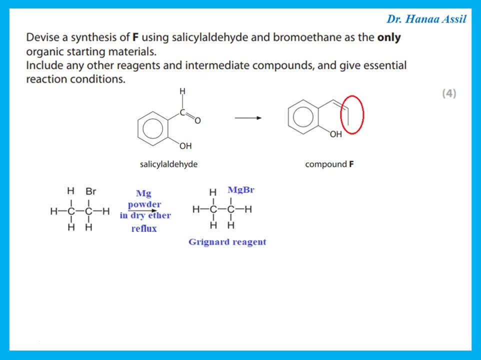 We're trying to add that group to it. So what's the first thing I can do? I can use greenery, So I can start with. he's saying: I can start with bromoethane, So I use the bromoethane to make a greenery reagent. 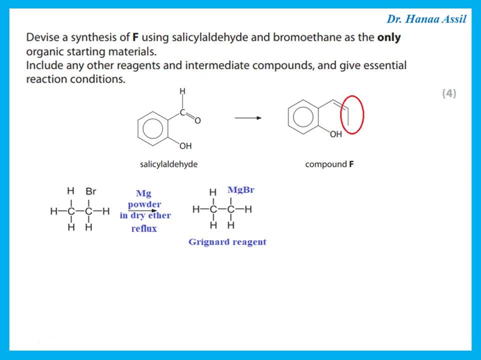 Remember Reacting the halogenoalkane with magnesium in dry ether Reflux. these are the conditions. I add magnesium bromide to the halogenoalkane So I prepared the greenery reagent. Then I need to add that group. 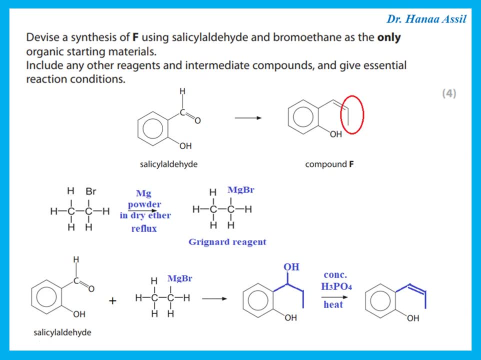 So I react this greenery reagent with the salicylaldehyde. This gives me that group added on the benzene ring. Now I want to remove the OH and put a double bond. So this is actually dehydration. So that is concentrated phosphoric acid and heat. 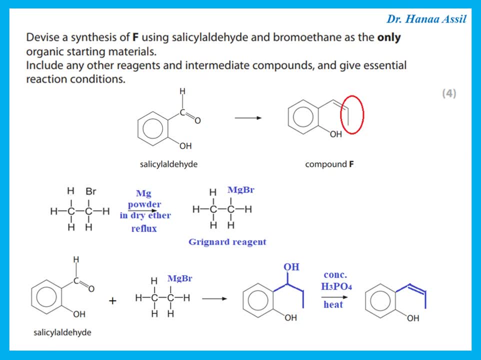 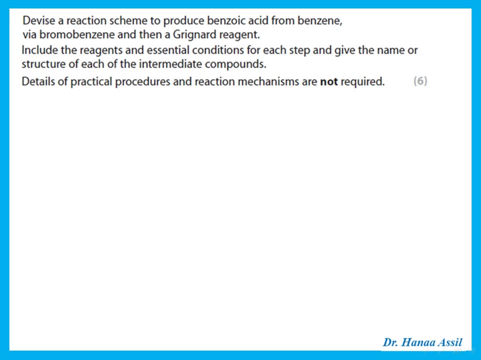 This gives me the product we're trying to make. Okay, This question says: devise a reaction scheme to produce benzoic acid from benzene via bromobenzene and then a greenery reagent. So we want to start with benzene. 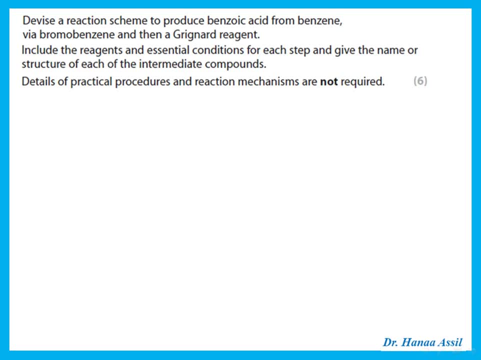 change it to bromobenzene, make a greenery reagent and then get benzoic acid. Include the reagents, essential conditions, the name or structure of each of the intermediate compounds. So let's take a look. We're trying from benzene. 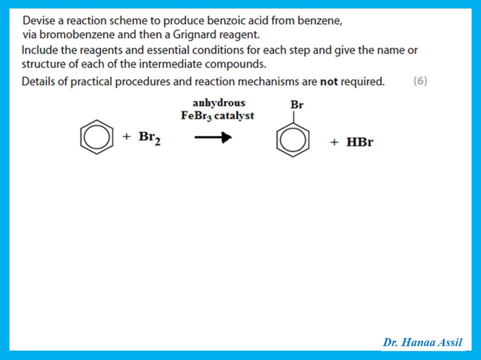 So I can use benzene to make bromobenzene. I'm adding, for example, bromine in presence of anhydrous FeBr3 as a catalyst. This puts a bromine on the benzene. Now I can use this to make a greenery. 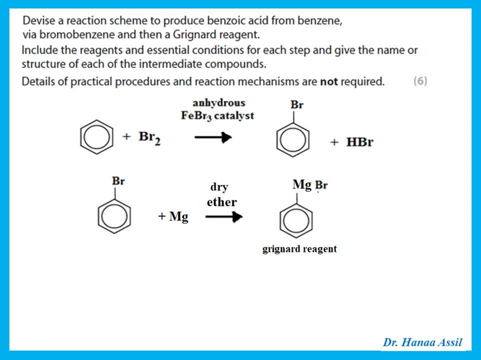 We said to make a greenery. We said we react it with what? Magnesium in dry ether? This gives me this greenery agent. Then I want to react it with what. to give benzoic acid? We said if we react the greenery with carbon dioxide. 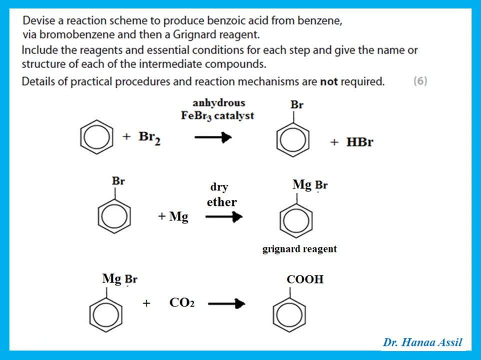 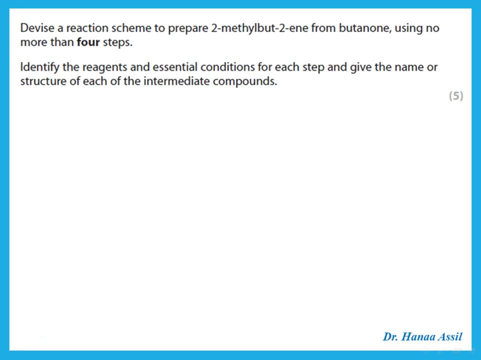 this gives a carboxylic acid on the benzene ring. Okay, Another question: Devise a reaction scheme to prepare. What are we trying to prepare? 2-methyl-but-2-ene-from-butanone. 2-methyl-but-2-ene-from-butanone. 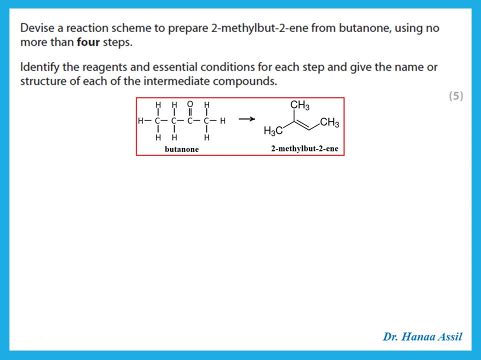 And he's saying: using no more than four steps, Identify reagents, essential conditions, name or structure of the intermediate compound. So we're starting with butanone. What can we do to change it to 2-methyl-but-2-ene? 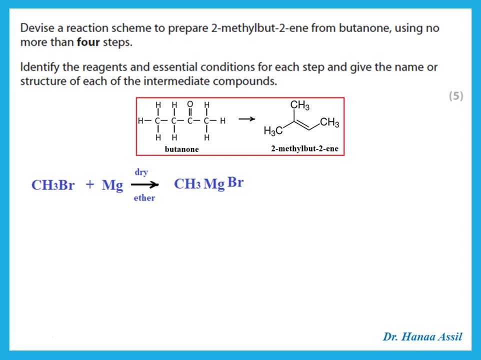 Okay, Let's start using. Remember that we're going to add a methyl group to the butanone. The butanone is something that has four carbons. We want something that has five carbons, So that means I'm going to use a green unit. 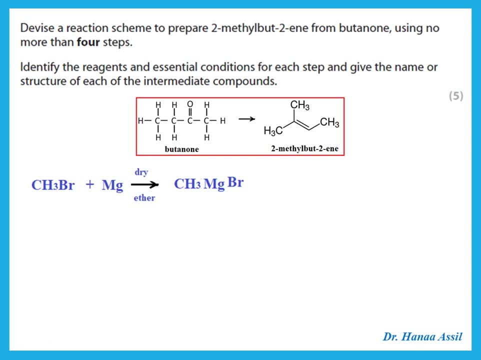 Now what am I adding? I'm adding that extra methyl group there. Now I make a green unit using methyl bromide magnesium in dry ether. I get the green unit reagent. Then I can react the green unit reagent with the butanone. 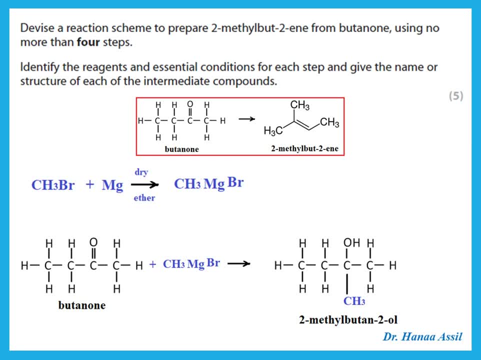 What will that do? That will add the extra methyl group on that carbon, But then I have it in the form of an alcohol. How do I change the alcohol into an alkene? Concentrated? Concentrated phosphoric acid will give the required product. 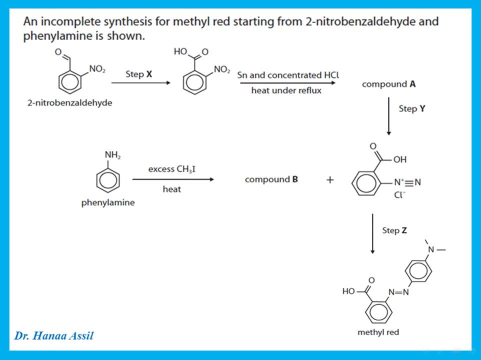 Okay. Sometimes he gives you the synthesis and asks you things about the synthesis. So let's take a look at this. He's giving me an incomplete synthesis for methyl red, starting from 2-nitrobenzaldehyde and phenyl amine. 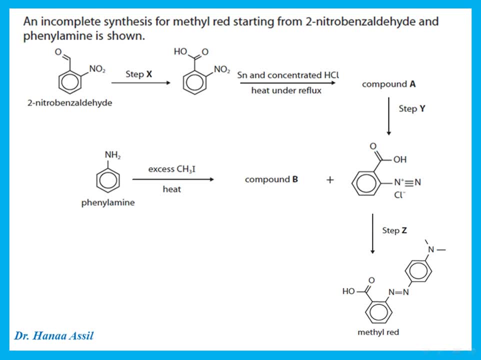 So I have the two compounds that I can start with, 2-nitro Benzaldehyde and phenyl amine, And in the end I want to get that compound at the bottom methyl red. Okay, From the nitrobenzaldehyde. what can I do? 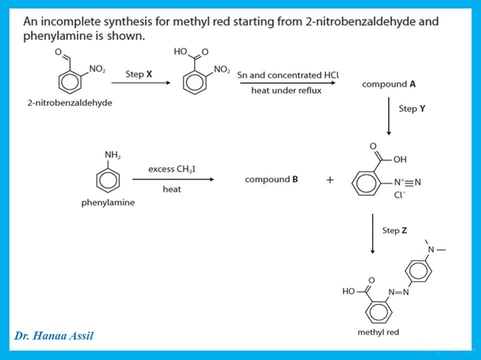 I can change the benzaldehyde to acid. So he's telling me This is something he gives me. He's changing the aldehyde first into acid. So what should we use? An oxidizing agent, of course, Like acidified potassium dichromate heat on the reflux. 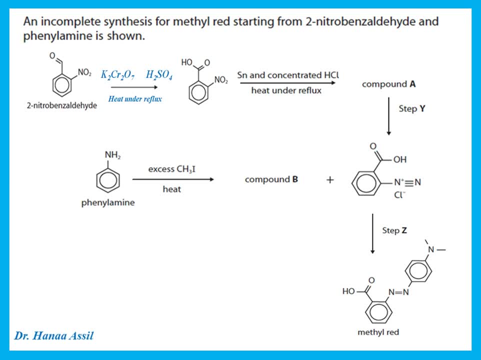 This will give the acid instead of the aldehyde. Then he's going to add tin in presence of HCl. What does that do? Remember that tin in HCl will change what. It will change that NO2 group to NH2.. So it changes the nitro to amino. 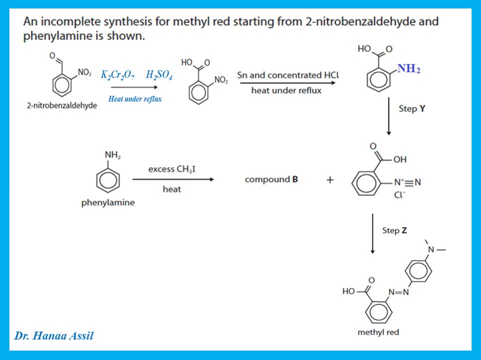 Then he wants to change that amino. He wants to change that amino group to a diazonium salt. What do we do to change an amine group to diazonium salt? React it with sodium nitrite plus HCl, So in that case we got the diazonium salt. 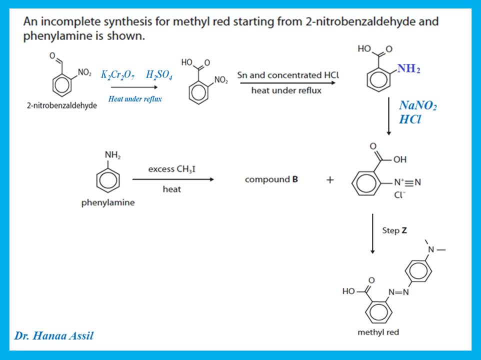 Now we want to react it with something to give the methyl red. So he got the phenyl amine. He added excess methyl iodide and heat. What happens if I add an alkyl halide to an amine? It replaces the hydrogens on the nitrogen to methyl group. 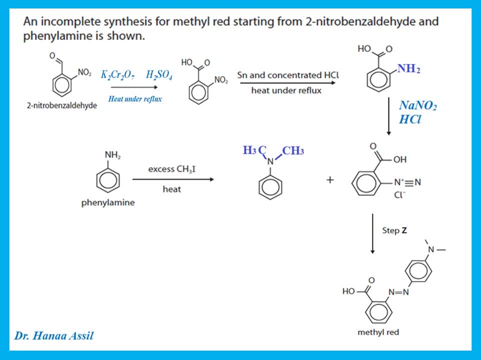 So he has excess. That means we're going to replace both hydrogens on the amine group with a methyl group. React these together. You end up with the compound that he's trying to make. Okay, Now, when we react them together, 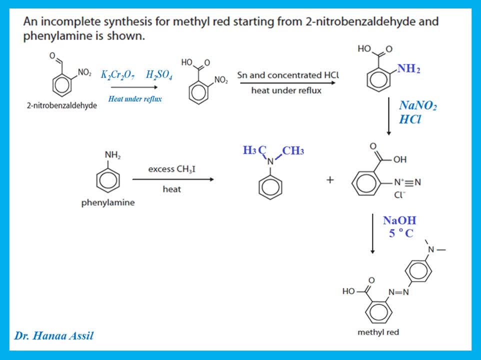 you have to know that this is, in alkaline conditions, A very low temperature. We said the diazonium salt needs a temperature less than 10 degrees Celsius or it will decompose. So this is the coupling reaction to give the methyl red. 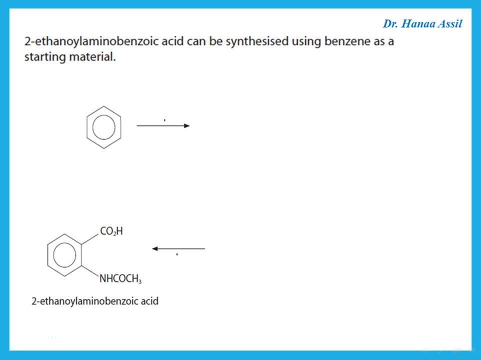 Another question. This was saying that he wants to react. This is saying that he wants to make two ethanoil amino benzoic acids And he wants to start with benzene. So what do we do to the benzene to end up with two ethanoil amino benzoic acids? 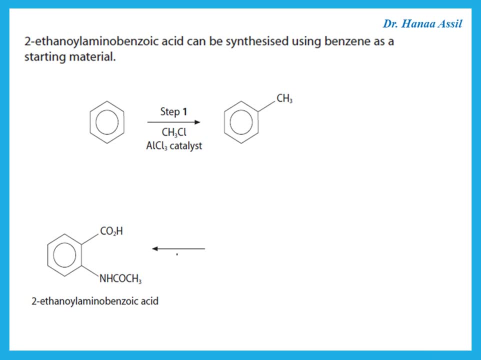 First, I can put a methyl group on the benzene ring. What do we do to put the methyl group on the benzene ring? React with methyl chloride in presence of aluminum chloride? Then what? Look at the final product and see what we can do. 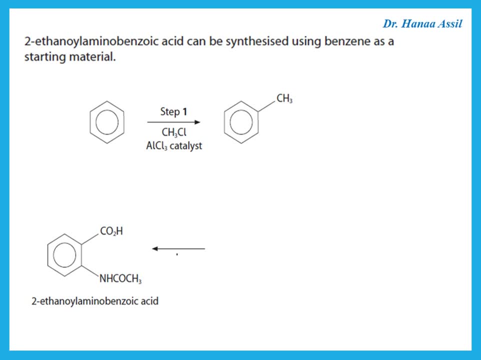 The next step. we either oxidize the methyl group there or we add that other group at the bottom. So in order to add that group at the bottom, I can add a nitro group. Remember to add the nitro group. we need concentrated nitric acid and concentrated sulfuric acid. 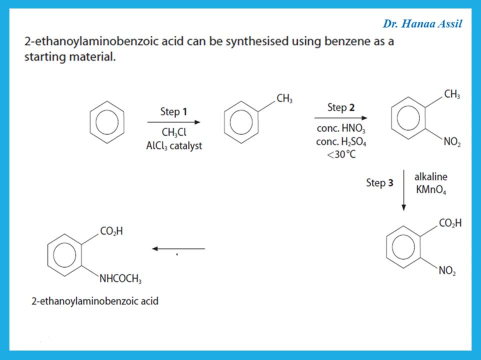 Then oxidize. I oxidize the methyl. I can put alkaline, potassium, manganate. It oxidizes the methyl on the benzene ring to acid. Now I want to change this group to what? To an amino group. So I'm going to change the NO2 to NH2.. 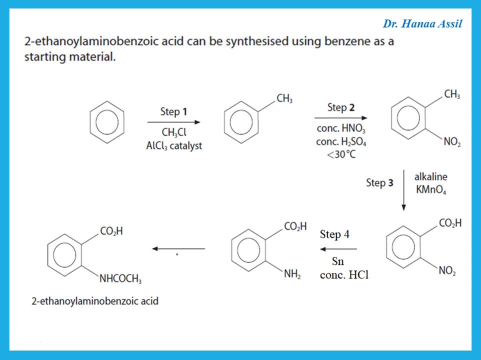 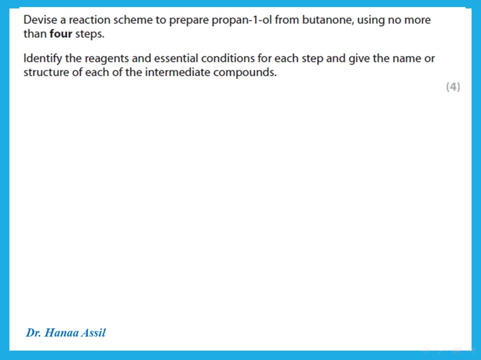 This uses what We use: tin in concentrated HCl. Then what do I do to get that final product? I react this compound with ethanoil chloride. This will give 2-ethanoil-amino-benzoic acid Okay. 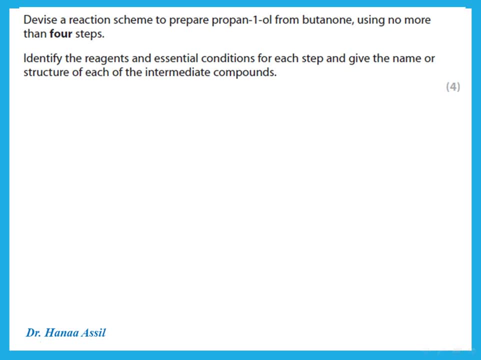 This question says: devise a reaction scheme to prepare Propane 1-ol from butanone. So we're trying to make propane 1-ol from butanone. Of course this means I'm removing one of the carbons of the butanone. 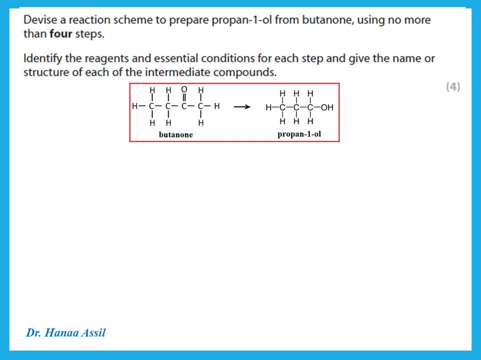 Okay, And he says using no more than 4 steps. So how do I change butanone to propane 1-ol? Well, the first thing I can do is remove the extra methyl group. Remember we said: if I have a methyl next to a ketone. 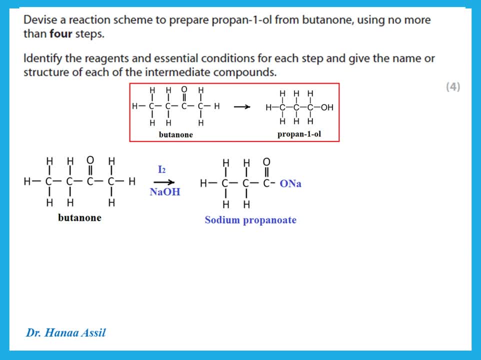 I can add iodine in presence of sodium hydroxide, alkaline iodine solution. It removes that extra CH3 and puts sodium salt instead of it. So this prepares sodium propanoate. Then what? I want to change that eventually to propane 1-ol. 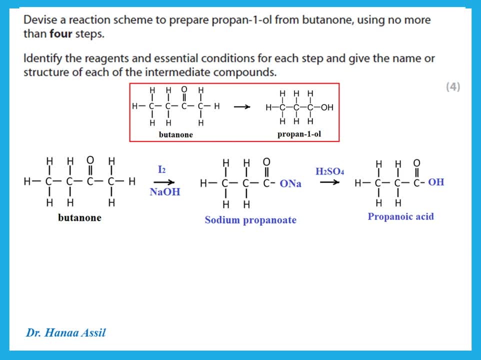 I can add. I can add acid in order to change the sodium salt to propanoic acid. And then how do I change propanoic acid to propane 1-ol? I just reduce lithium aluminum hydride in dry ether will give the required product. 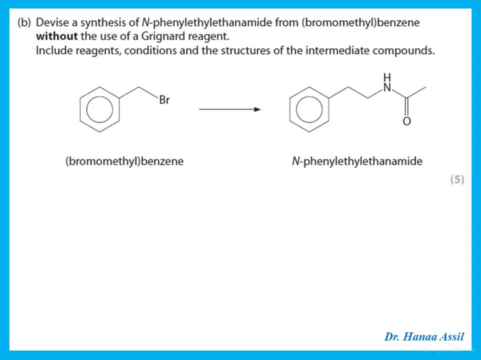 Again. let's try this. He's trying to devise a synthesis of this final compound, N-phenyl ethylethanamide, starting from bromomethylbenzene, And he's specifying without- please note the instructions- without the use of a greener reagent. 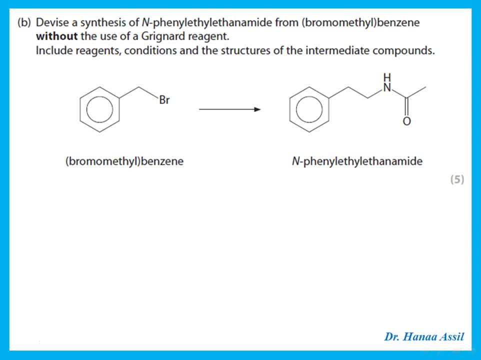 So we're not going to use greener here, And I want to change bromomethylbenzene to that final compound. So what should we do? Well, let's see. First, I can change this into a nitrile group. 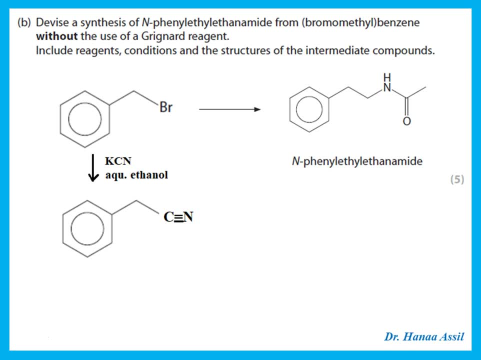 Remember. this will help me to add an extra carbon on the chain. How do we do this? We reacted with potassium cyanide in aqueous ethanol. You replace the Br with the cyanide or the nitrile group, Then what? Then we can reduce this lithium aluminum hydride in dry ether. 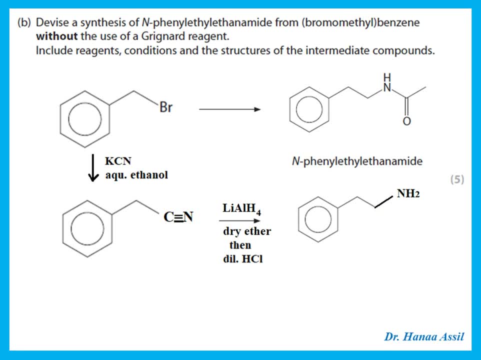 This changes it to an amine with an extra carbon. So now we have added an extra carbon to the chain and we have an amine. Now how do we change it to that final compound? I can just react it with ethanol chloride. 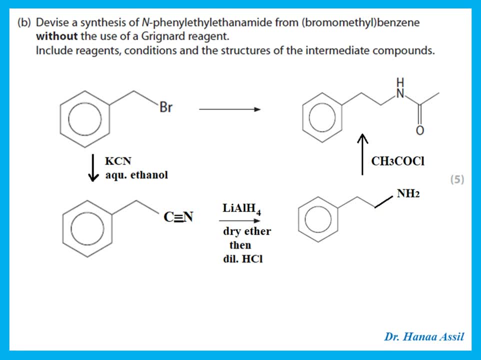 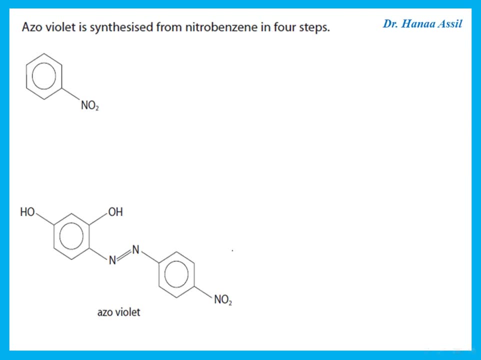 This will add the required chain to the amino acid Chain to the amino group, And that gives me my product Again. let's try this. He's trying to make azoviolet- Can you see azoviolet? And we want to start from nitrobenzene in four steps. 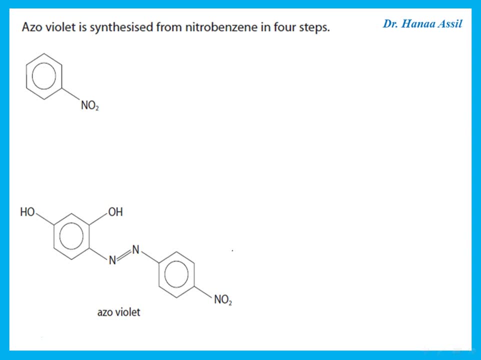 So nitrobenzene? Look at what you're starting with and look at the final product and see what we're trying to add. Can you see the nitrobenzene? Obviously, we need to make a diazonium salt and then react it with that other one. 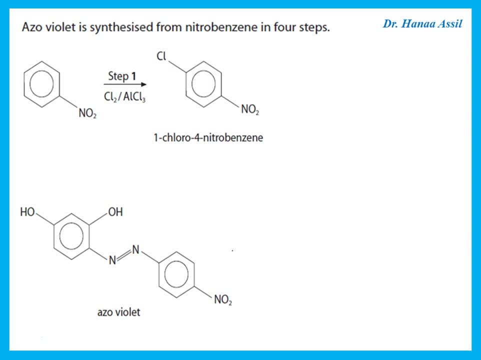 So let us see what we should do. We add a chlorine on the benzene ring, So we react this with chlorine in presence of aluminum chloride. This gives me the chlorine on the carbon number four of the benzene ring. Then I can change this chlorine to an amine group. 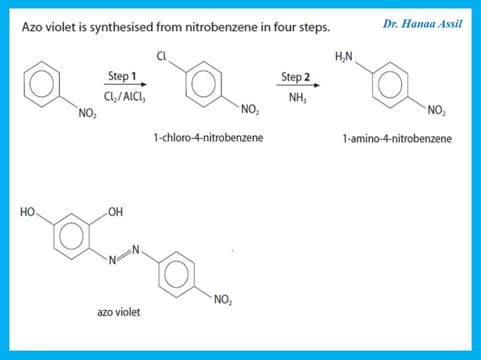 So I react it with ammonia. It replaces the chlorine on the benzene to an amine group. Then what? Then I can change that amine group into the diazonium salt. So we add sodium nitrite in HCl, or basically reacting with nitrous acid at low temperature, less than 10 degrees. 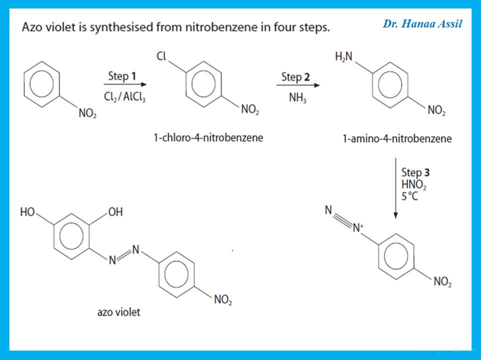 This gives me the diazonium salt. How do I change this diazonium salt to my final product? I have to react it with this part of the compound. So that is the part we're adding And of course, this coupling reaction is in presence of sodium hydroxide at five degrees Celsius. 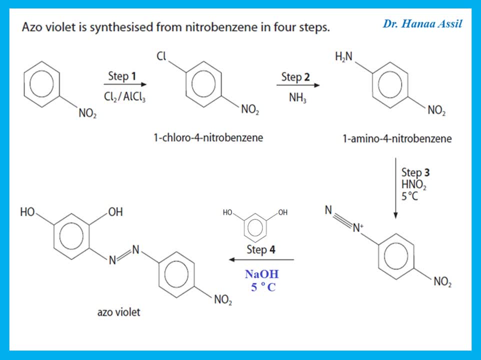 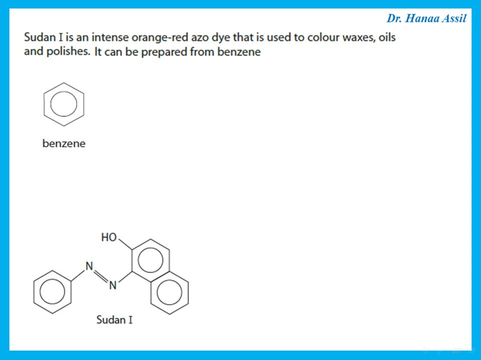 This gives me my final product, Another synthesis. He's trying to make something called Sudan-1. And he's saying it's an intense orange-red azo dye that is used in color waxes, oils and polishes, And we need to prepare it from benzene. 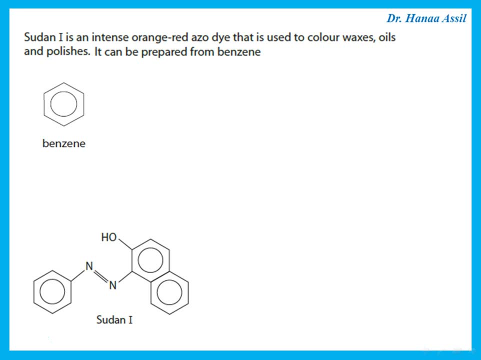 Can you see that? Okay, So what do we want to do? First, add a nitro group on the benzene ring. React with concentrated nitrate, concentrated sulfuric and heat. This puts the nitro group on the benzene ring. 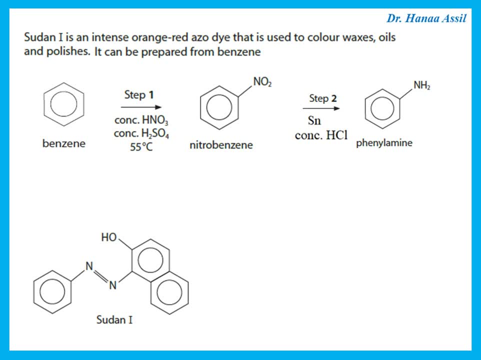 Then reduce that to the amine using tin in concentrated HCl. So this puts my amine group on the benzene ring. Then I need to make the diazonium salt, So I react it with sodium nitrite, HCl at five degrees Celsius. 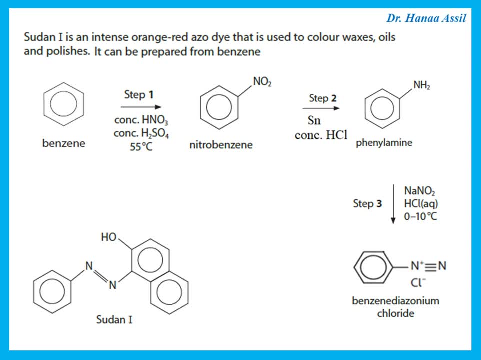 This gives me the benzene-diazonium chloride. Then what? And then I want to add that extra group to the diazonium salt. That means I'm reacting it with this Again, in presence of sodium hydroxide: five degrees Celsius. 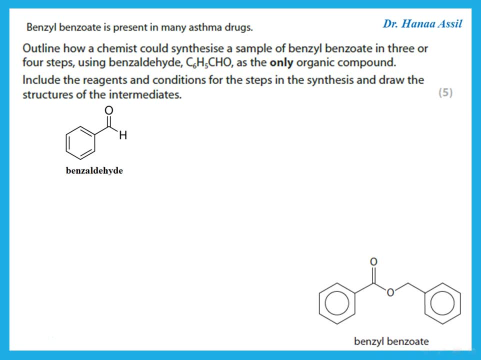 And I get my product Benzyl benzoate. Can you see what is benzyl benzoate? That's my final product down there. It's present in many asthma drugs. Outline how a chemist could synthesize a sample of benzyl benzoate. 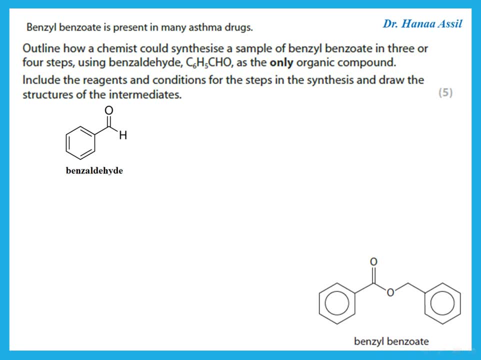 In three or four steps, Using benzaldehyde as the only organic compound. Include reagents, conditions and structures of the intermediate. Okay, So I'm starting with benzaldehyde And I want to end up with that benzyl benzoate. 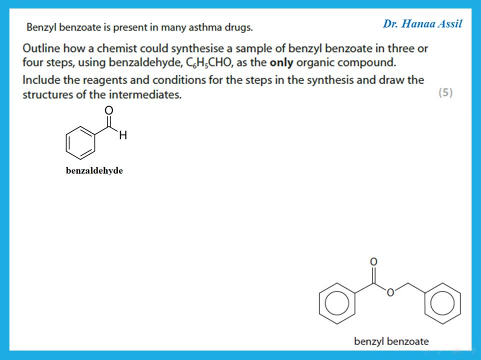 So what's the first thing I can do? Well, I can oxidize the aldehyde to acid. Sulfuric acid and potassium dichromate will oxidize the aldehyde to acid. Then what This benzaldehyde I can also use to make. 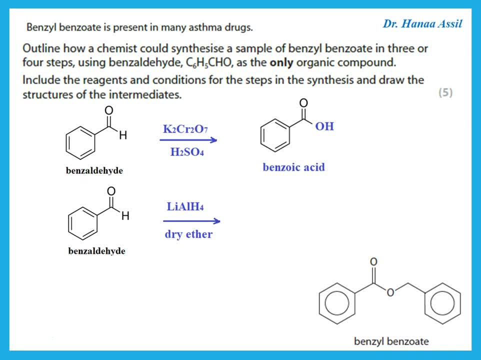 Remember that he's saying: benzaldehyde is the only organic compound that I'm starting with, So I have to change this benzaldehyde to that other product that I'm trying to make: Lithium aluminum hydride in dry ether will change the aldehyde to alcohol. 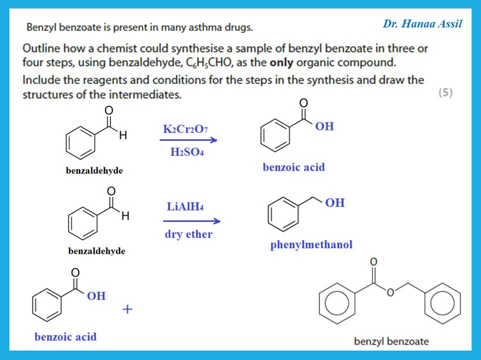 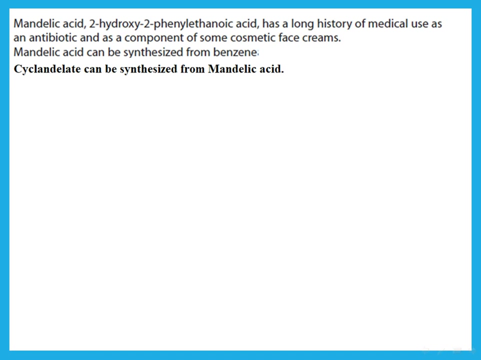 And then this benzoic acid reacted with the alcohol in presence of concentrated sulfuric acid. So this is basic esterification. will give me the benzyl benzoate. Are we okay with this? Another synthesis: He's saying mandelic acid to hydroxy, to phenyl ethanoic acid. 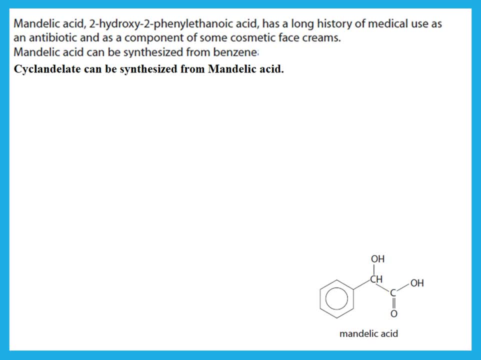 This is mandelic acid And he's saying it has a long history of medical use as an antibiotic and component of face creams and so on. And he's saying mandelic acid can be synthesized from benzene, So we're going to start with benzene. 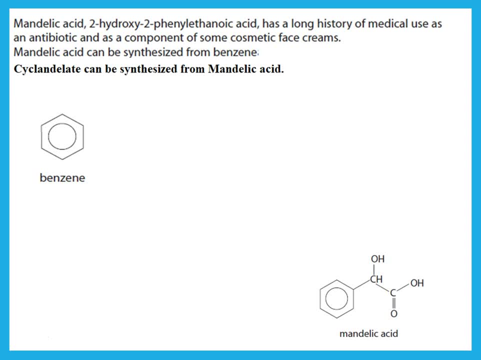 Make mandelic acid. And then there is another compound. This one, which he calls cyclandelate, will be synthesized from mandelic acid. So let's go through this: Starting from benzene, I want to make mandelic acid, and then that final product. 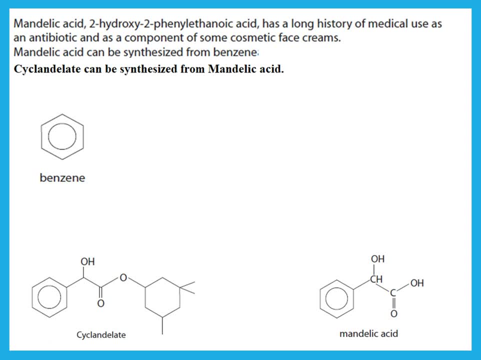 So what can I do? What did he add on the benzene ring to make the mandelic acid? Well, we can start with adding an aldehyde group. So adding an aldehyde group is methanoil Chloride in anhydrous aluminum chloride. 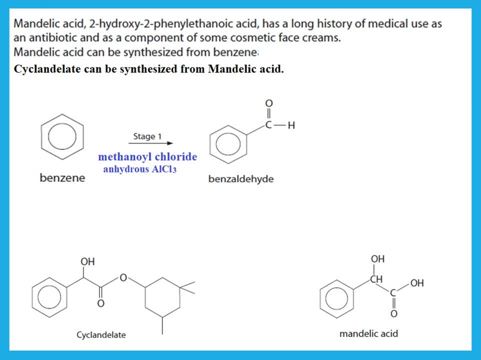 That will add aldehyde to the benzene ring. And then what? And then I'm going to add: remember, I need to add extra carbon, So I need to react it with potassium cyanide in HCN. This will change the aldehyde to a nitrile group. 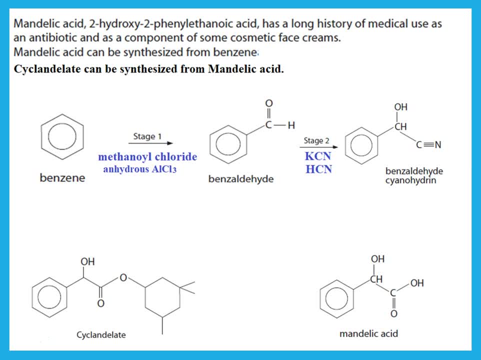 So I'm adding an extra carbon here, Then what? In presence of acid that will hydrolyze the nitrile group. So I get an acid with an extra carbon, So that is my mandelic acid. Then what? In order to get that final product? 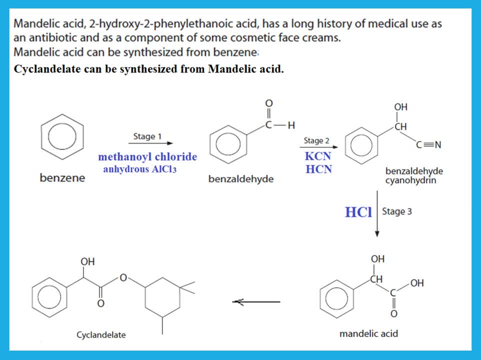 Can you see what it is? This is just an ester in which you're adding that group to the acid. This will give you the ester To the ester that he wants. Of course, esterification is in presence of concentrated sulfuric acid.